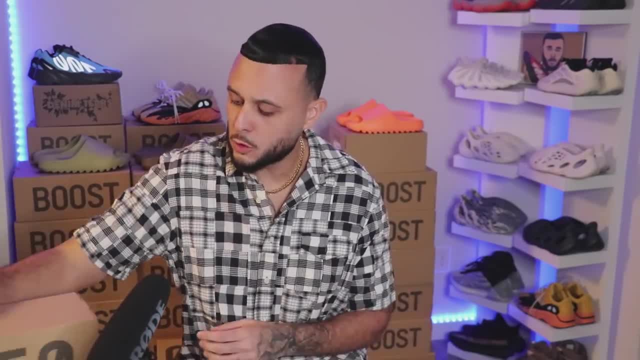 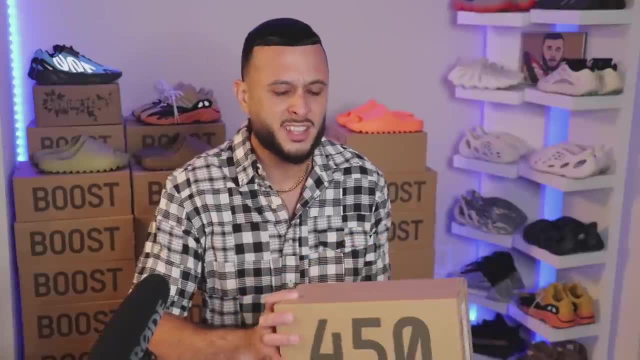 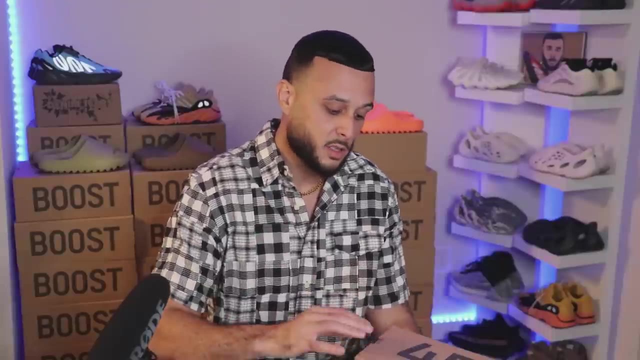 are game changers on the market. So the Yeezy 450 was teased to us for some years. What really draw people towards the silhouette, I gotta say, is the sole. We then saw Yeezy debut these during Paris fashion week a couple years ago and the hype has been crazy ever since. So they finally 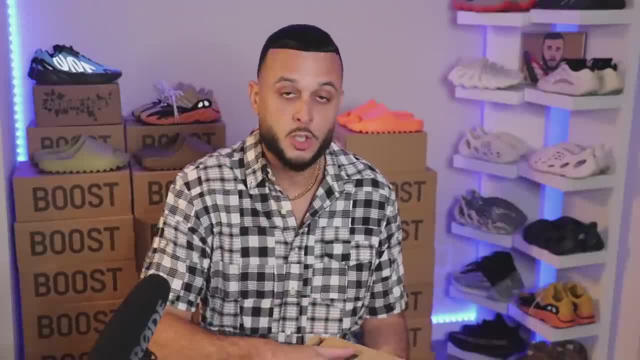 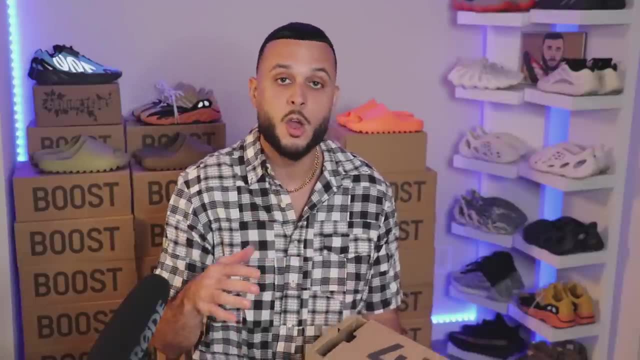 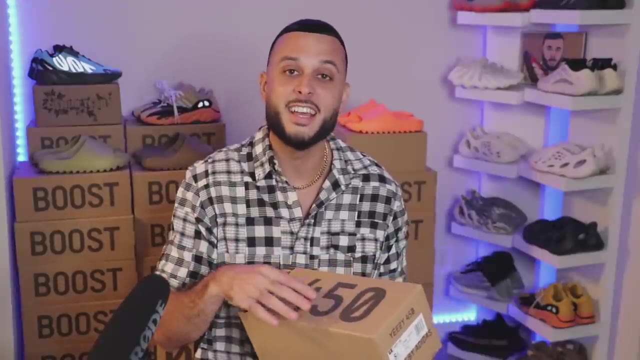 debuted, like we said, in March with the cloud white, So these dark slates will be the follow-up to one of the most hype Yeezy drops of the year. So what I need everybody to do, we're going to unbox these joints together and then I need you guys to drop your first impressions in the comment. 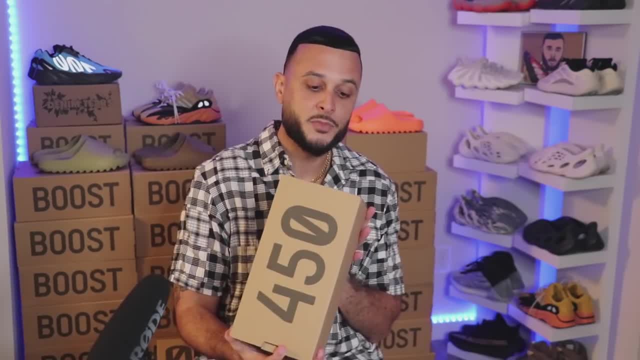 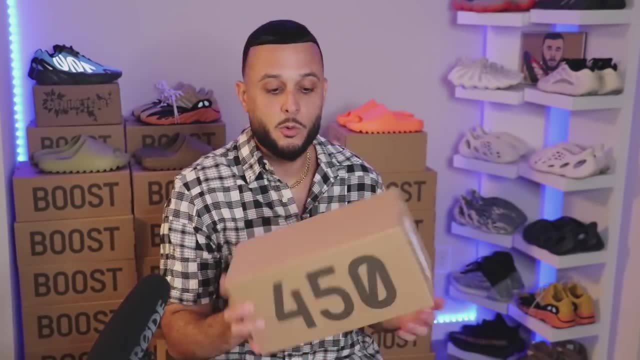 section down below. So make sure you guys smash the like button. We got the Yeezy dark slates which are made in Germany. Unfortunately these are not my size, so we will have somebody try these on so we can see an on-foot look, But I'm not sure if these are a must-have for my collection, you know. 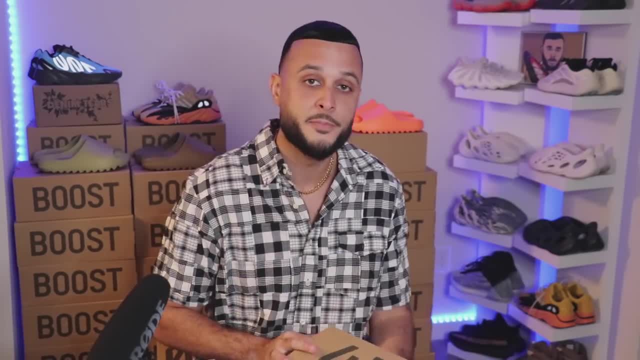 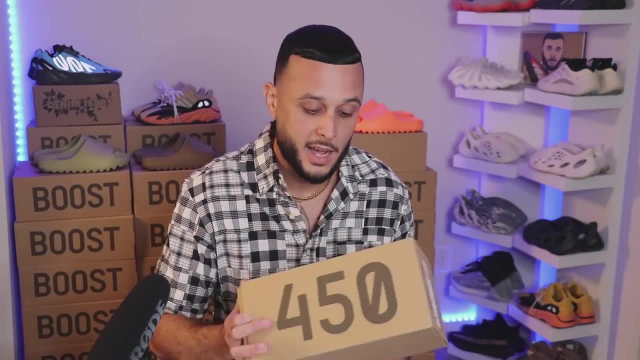 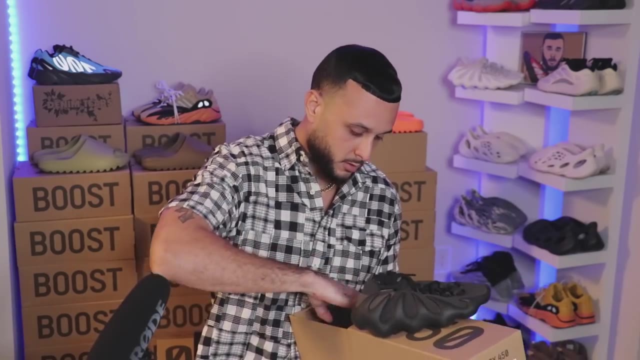 You guys already know how I feel about dark shoes. Sometimes I feel like they're unnecessary. I bought the 700 V3 Alva last year and they kind of just collected a lot of dust, so I'm not too sure about these guys. So smash the like button, Okay. so we got the Yeezy 450 dark slate guys, Y'all. 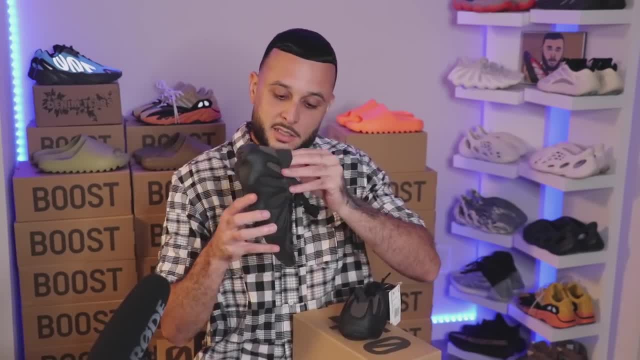 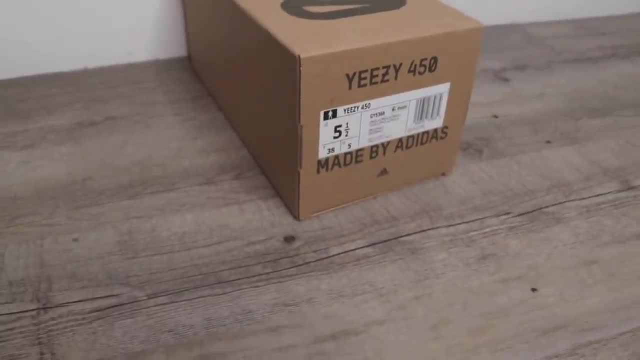 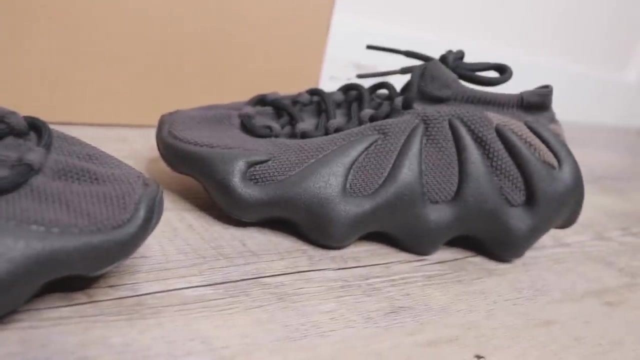 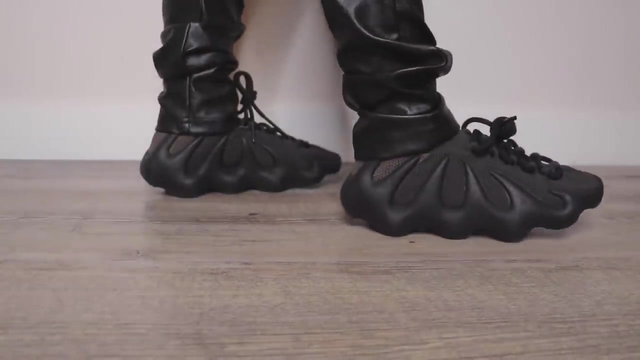 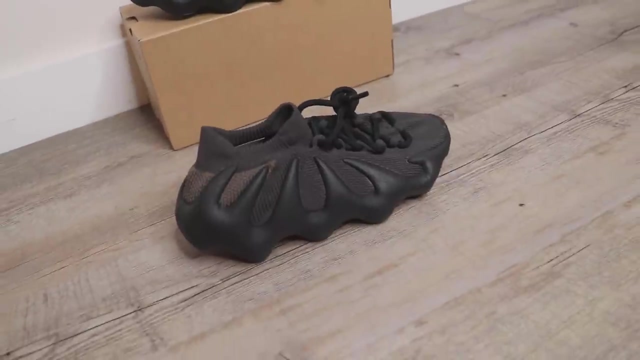 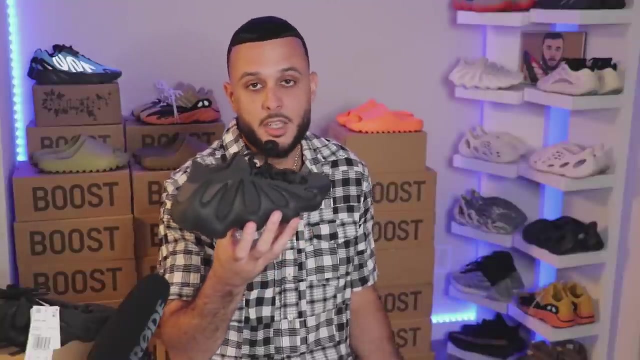 already know what time it is. man, Drop your first impressions in the comment section down below. So yeah, you pretty much got an all-black 450.. The only thing that's different is that it's got a detail. you'll notice, guys, It's some discoloration on the back heel area, So it's a faded black. I. 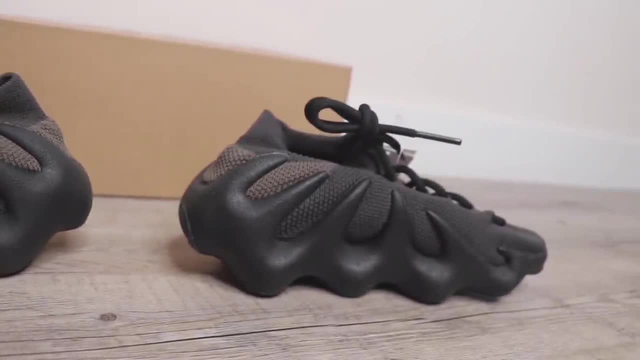 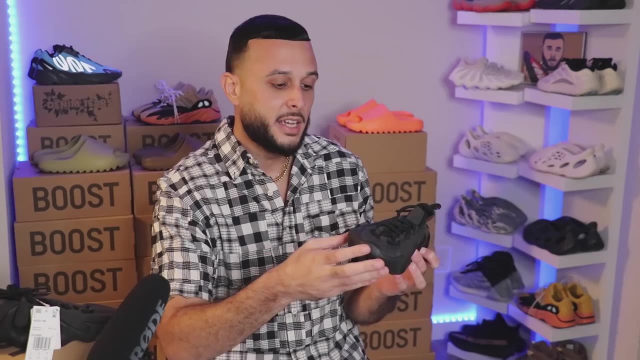 want to say. it's almost like someone took the back of this heel and just dipped it in bleach, So that detail doesn't really do anything for me. I think the real appeal of this sneaker is just the overall shape of this shoe. In my opinion is the quintessential travel shoe. 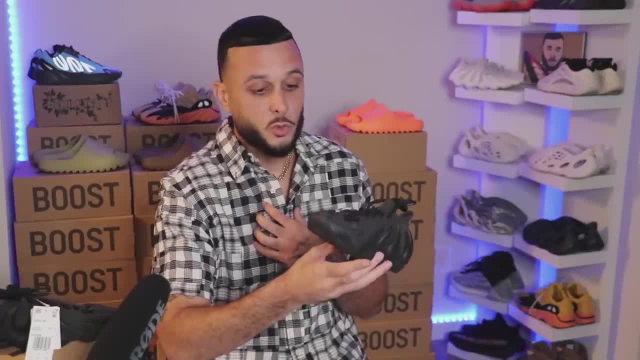 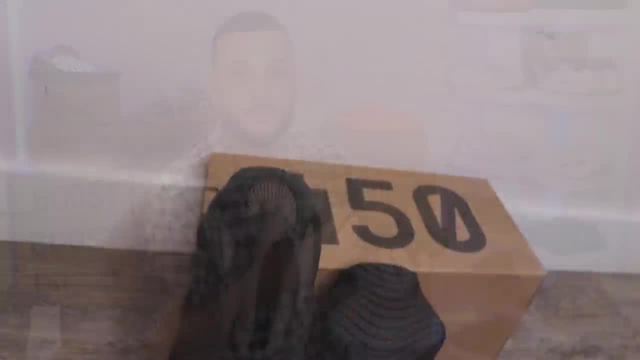 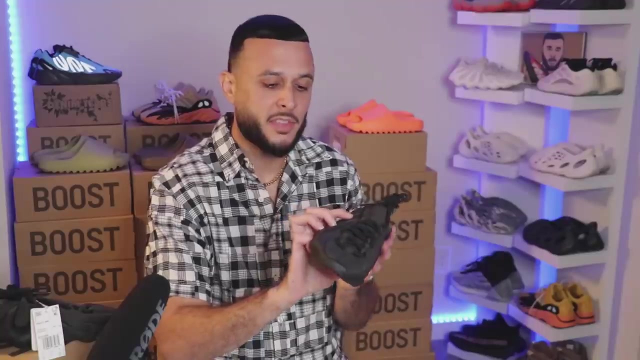 And with this sock-like upper, for me it's really replaced the 350. Literally like a sock with a sole engulfed around it. So while I'm usually not a huge fan of all-black sneakers, I really like these joints a lot. I think it's just the shape, The fact that it's a new. 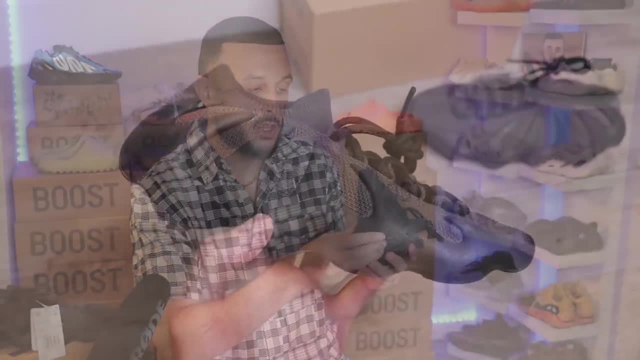 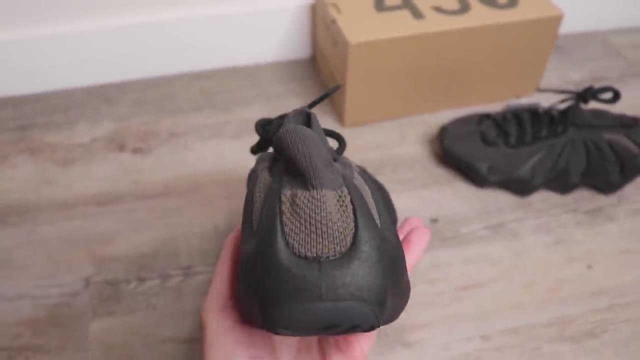 silhouette. I'm just really captivated by this sole And I want to say, with the black knit upper it works well And I'm just loving the way that this sole just engulfs the shoe. In terms of comfort, guys, I feel like the 450 is up the par. 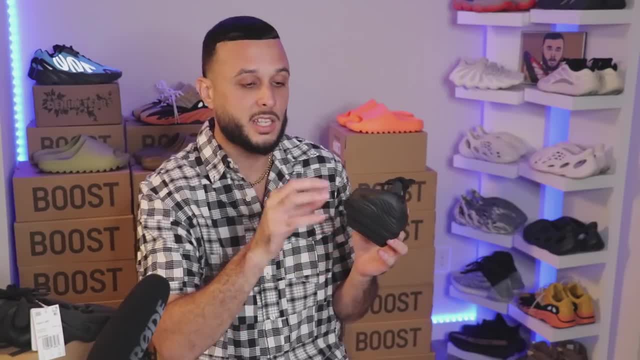 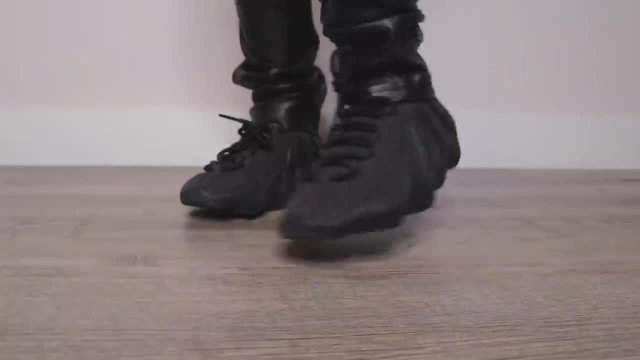 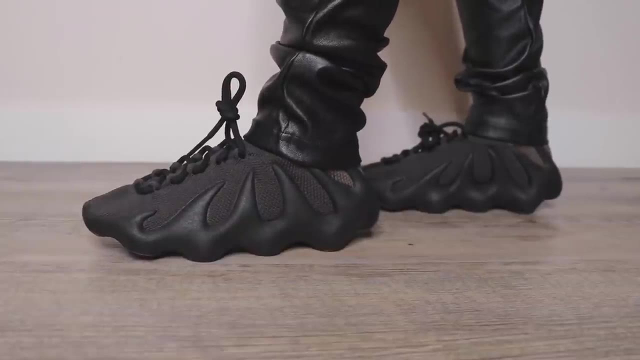 Just like we expect when it comes to the Yeezy brand, The technology used here is an injected EVA foam, So similar to what we have with the Yeezy slide. Now, the sock-like upper- knitted upper- of this sneaker really hugs your feet. So in terms of sizing, I would suggest to at least. 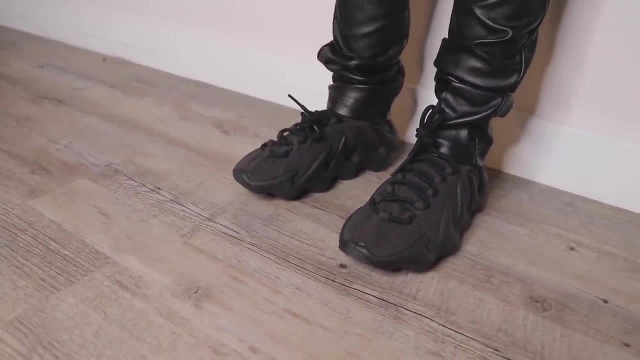 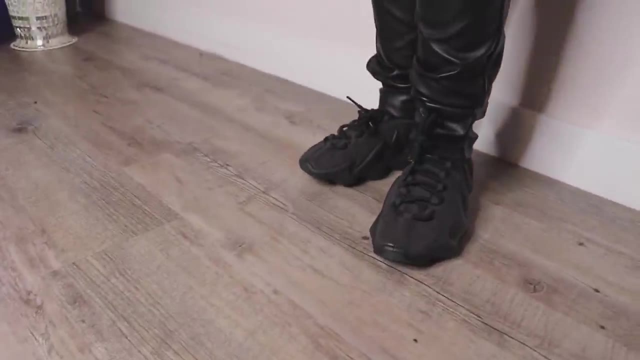 half size up. If your feet run wide, you definitely want to full size up As, like I mentioned before, the knitted upper is very tight, fitting towards your feet. So, with that being said, the tight-knitted upper really defeats the purposes of having laces. 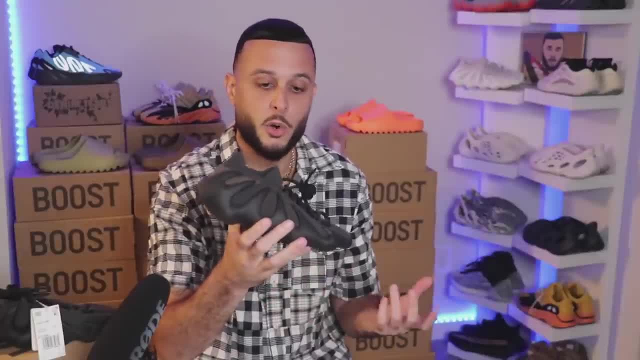 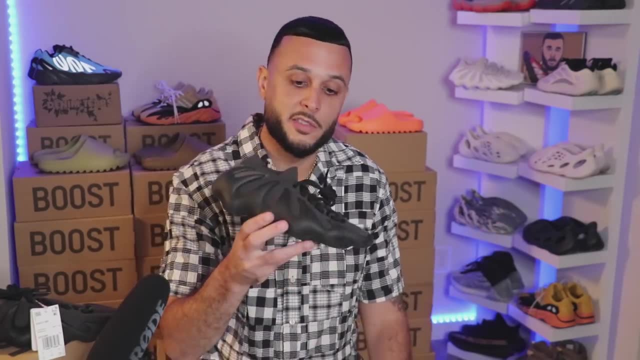 And I feel like it doesn't do much, as the sneaker already supports your feet. The laces really are just there to be aesthetically pleasing. in my opinion, This low-key may even be one of the last new Yeezy releases that features traditional laces, as Yeezy is innovating the game. Another. 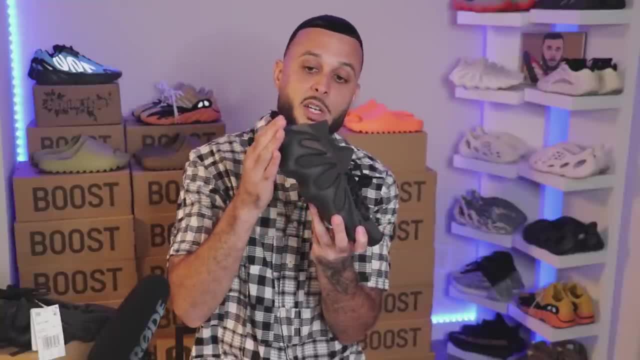 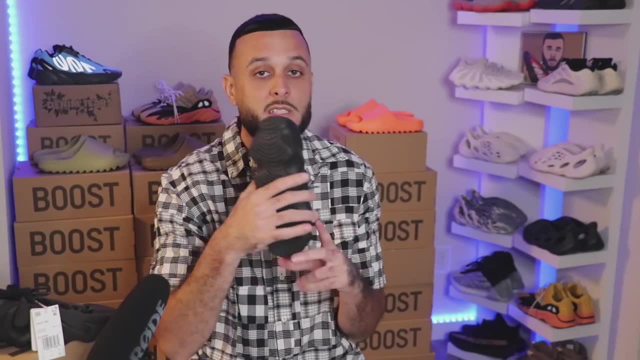 feature that you guys will notice is the elevated heel tab, which, in my opinion, it definitely adds to the level of comfort, And I think it's going to be one of the things that I'm going to be looking forward to. This is a feature that we've seen on a few different Yeezy silhouettes from the 700 V3. 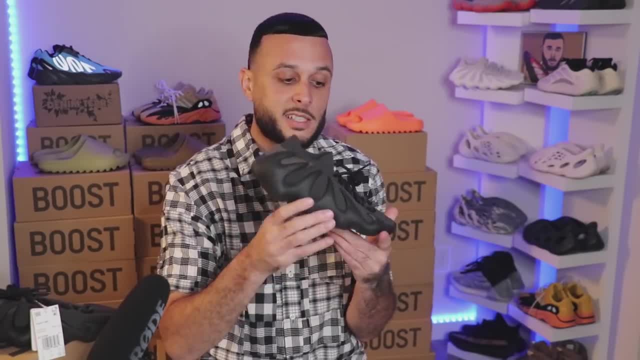 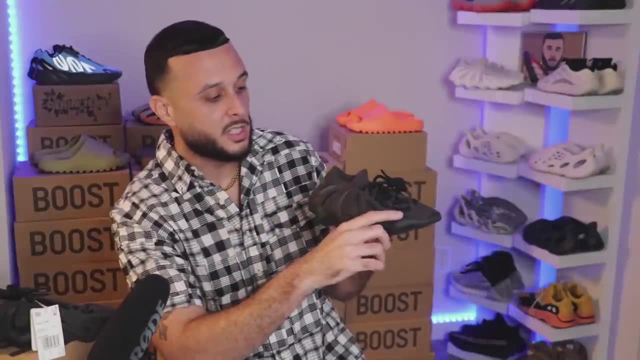 to the 380, as well as the Yeezy foam runner. Now, on this size, which is a five and a half, I want to say that everything size six and under will have six of these little fangs that you see here, while the larger sizes will feature seven. So for me, I actually kind. 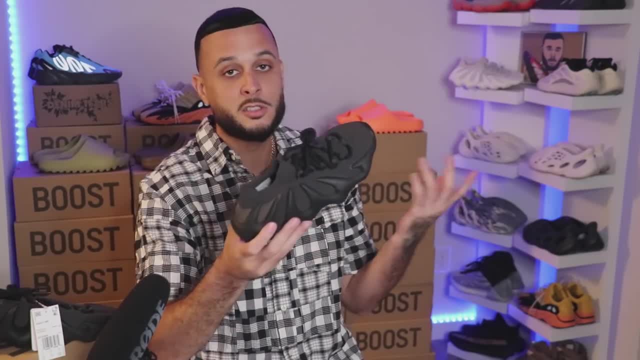 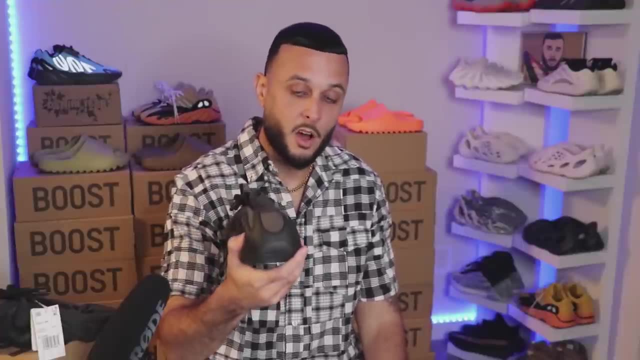 of like the smaller shoe, as the compact version of this shoe to me is more appealing. Now the final verdict on the 450. Speaker 1. The 450 Dark Slate is that although it is a black shoe, I'm just so in love with this. 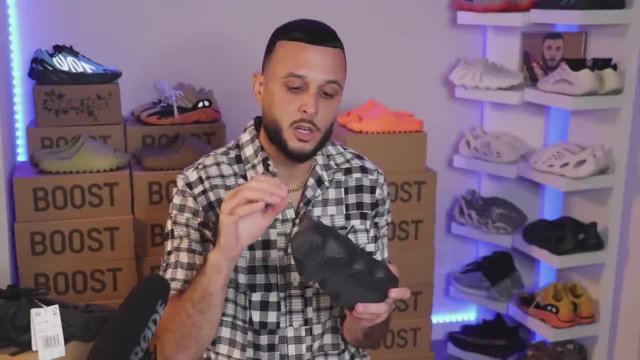 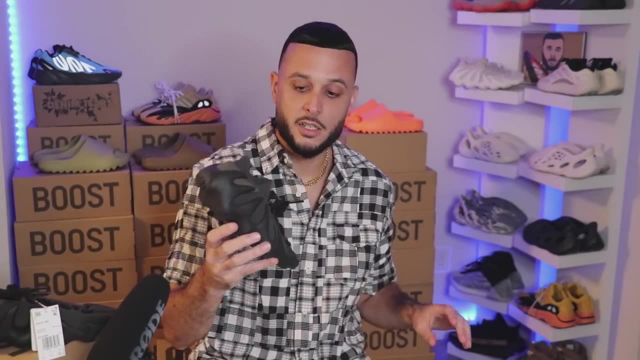 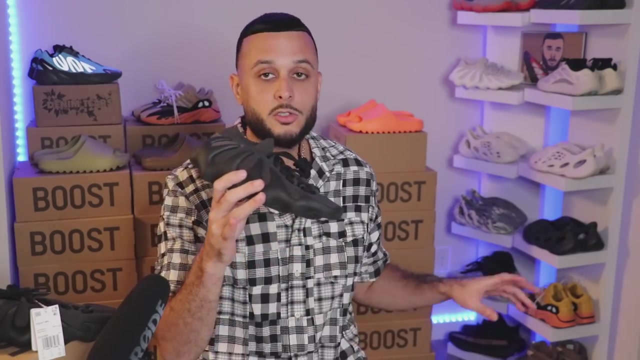 silhouette And I feel like with the knitted upper it really works well in terms of the color blocking. So for me these joints are a must have for the collection. I'm not so sure on what Yeezy has planned for the future for the 450, but I just kind of love the single tone. So 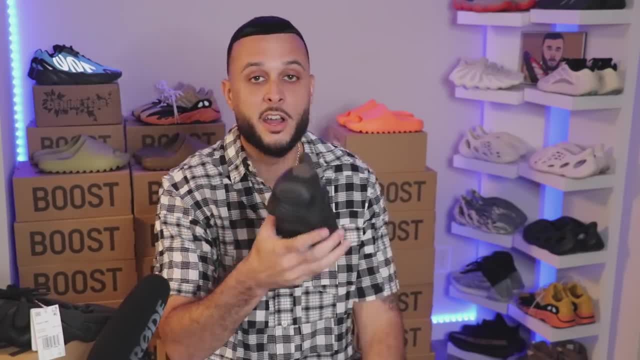 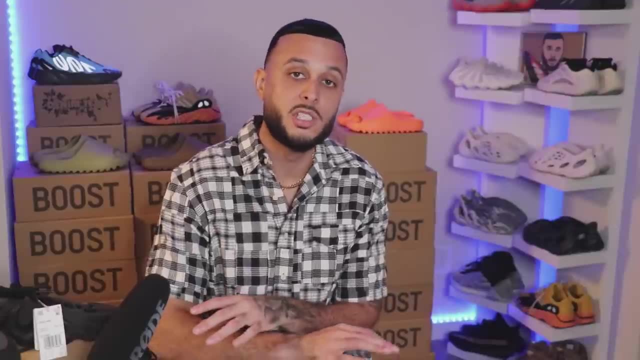 of course, the cloud whites dope, Dark Slate's dope. Really curious to see what the brand has in store for this silhouette Speaker 1. So earlier in the video I asked you guys if the month of June was even messing with the month of March in terms of Yeezy releases. If you guys recall, back in March we had a 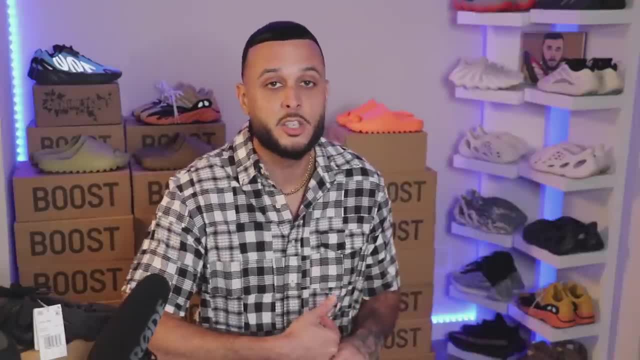 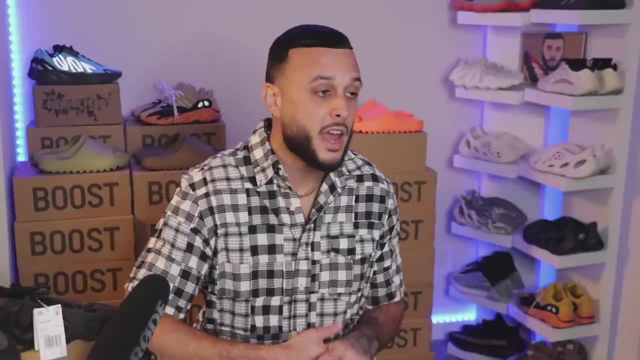 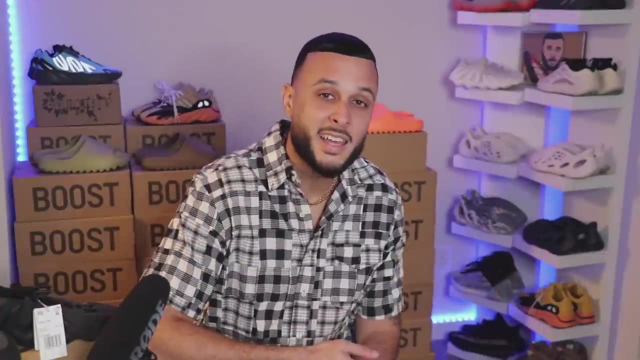 lot of heat from the 450 cloud whites. We had the 700 V2 creams. We had the foam runner sand, as well as the foam runner MX moon gray. We also had the desert boots and some more that I'm probably forgetting. So think about it. What about March? We had the bright cyan. 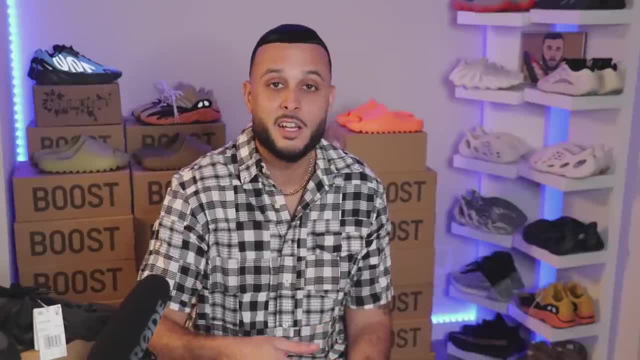 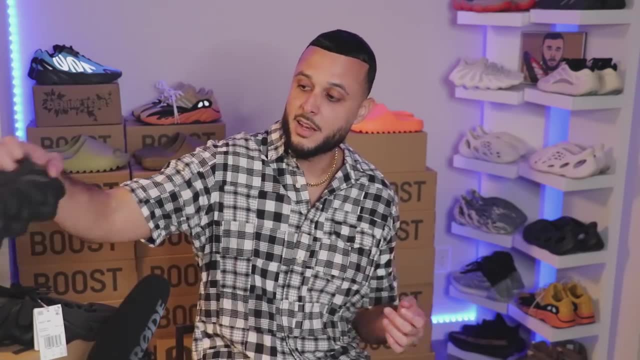 We had the taupe light 500s Speaker 1.. We had the 700 V1 inflamed amber orange slides, as well as some restocks of some previous colorways And now the 450 Dark Slate. If you guys ask me, June is right behind March in terms of releases. 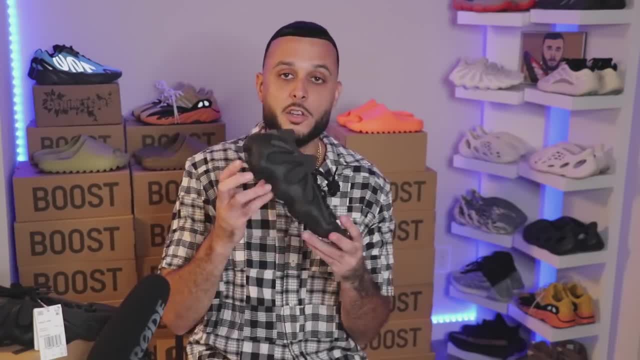 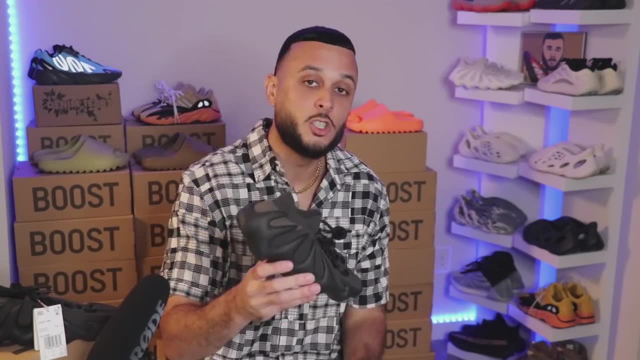 but let me know what you guys think in the comment section down below. Are you guys going to be picking up the Yeezy 450 Dark Slate which are rumored to be dropping, coming up this Friday, June the 25th, retailing at $200 US for $500. 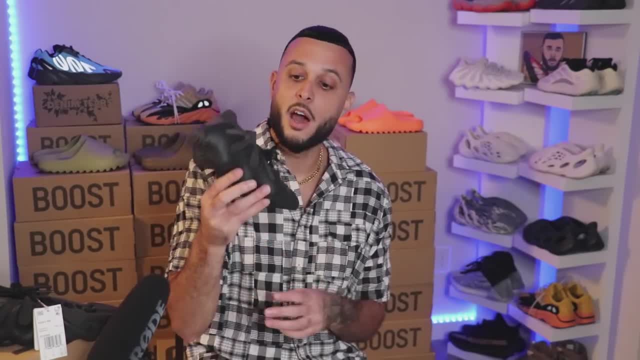 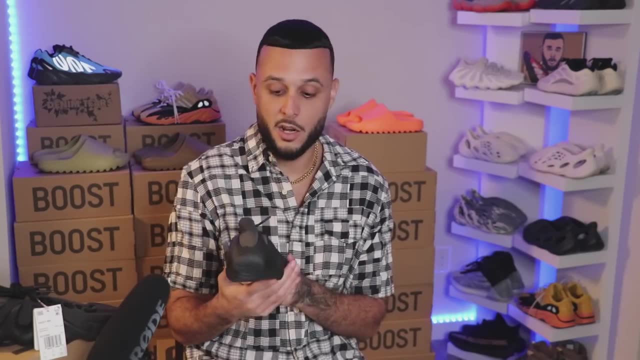 Speaker. 2. Speaker. 1. Speaker. 2. Speaker. 1. Speaker. 2. Targ to switch in August for adult sizes. they will be available in full family sizes. but, guys, this release is going to be a very hard cop, As you all already know. resellers-scalpers will be out to get these and the 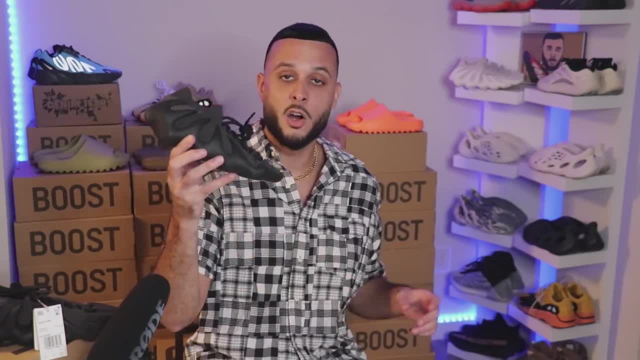 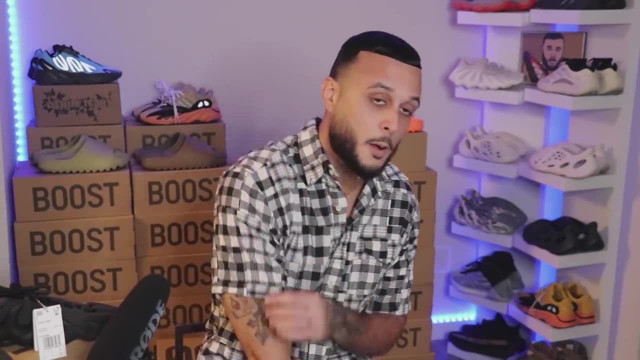 demand will be very high, So good luck to everybody. let me know if these are a cop or a drop. appreciate everybody for tuning in for today's video. I'm JA. stay safe, stay blessed, and I'm out. y'all Salute. 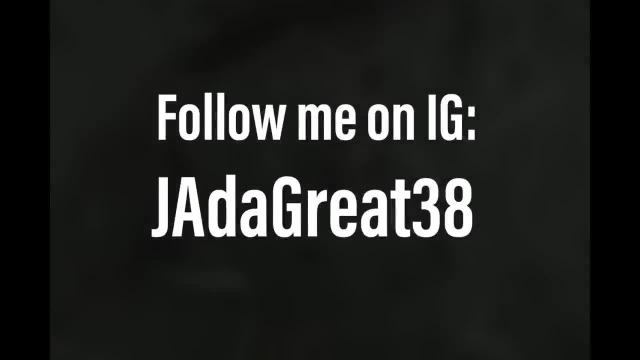 Speaker: 2. Speaker, 2. Speaker, 3. Speaker, 2. Speaker, 3. Speaker. 2. Speaker. 1. Speaker, 2. Speaker, 3. Speaker. 3. Speaker. 1. Speaker, 1. Speaker 2.. 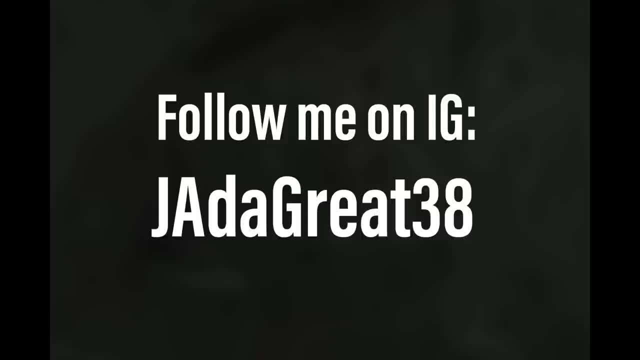 Speaker: 2. Speaker. 2. Speaker. 1. Thanks for watching.